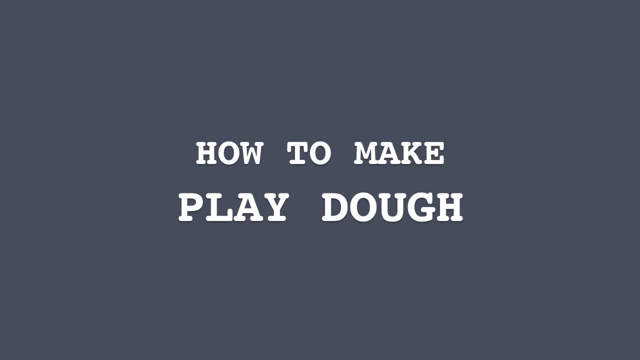 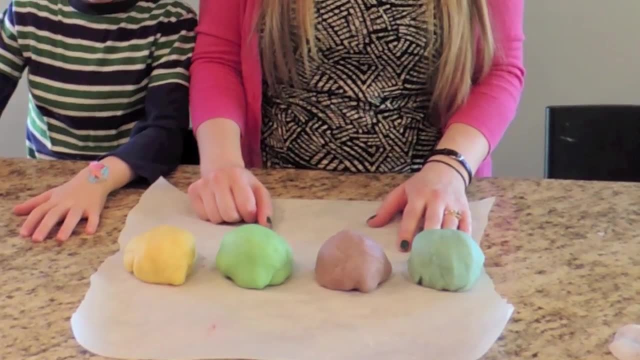 Hey, it's Kirsha Lee from Moms Have Questions 2.. Today, I'm going to show you how to make Play-Doh. Okay, this is, by the way, my personal favorite Play-Doh recipe. If you live in a 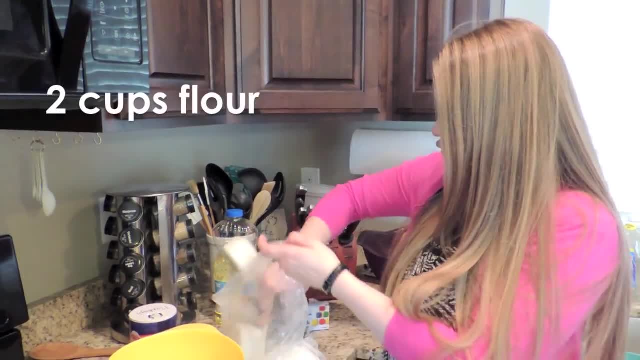 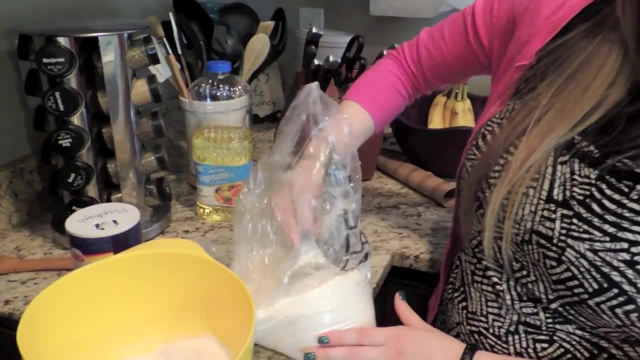 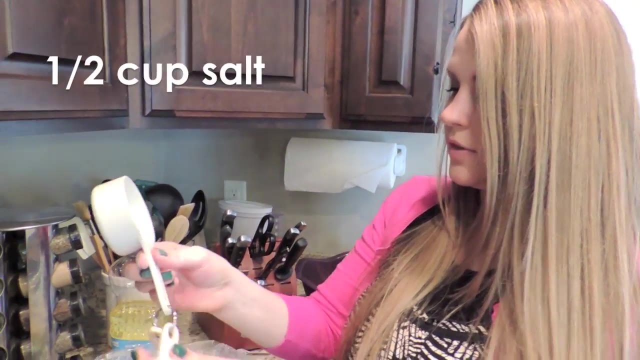 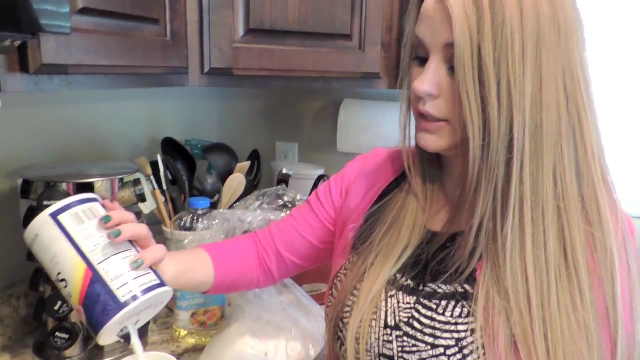 dry climate, I would suggest this one. Okay, so you get two cups of flour, One Two, Then a half cup of salt. Notice, the salt to flour ratio has a pretty low amount of salt. I think that's why it works so well for a dry climate, is that there's not very much salt, which 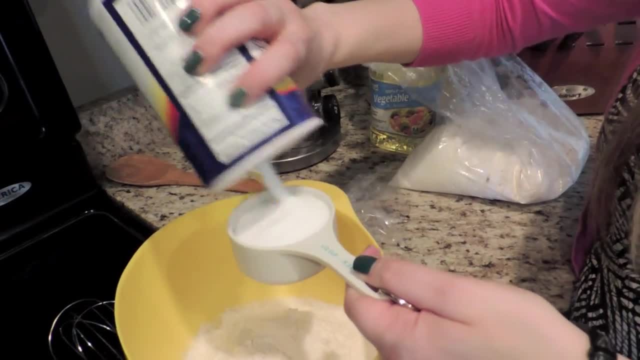 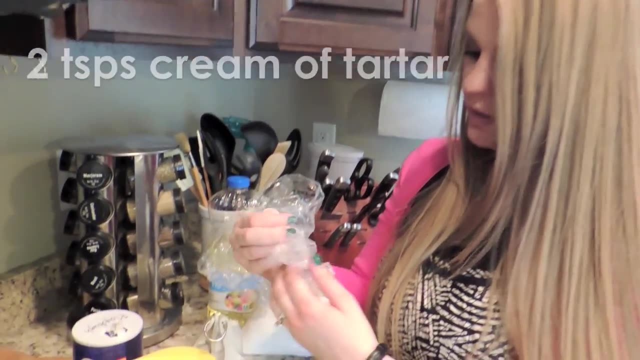 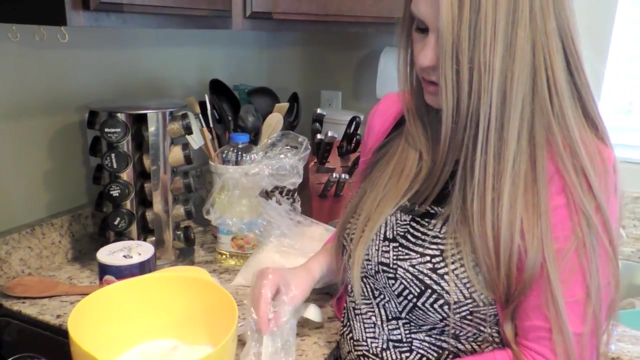 I love, because otherwise our Play-Doh dries out really fast. So this stuff is great. And then two teaspoons cream of tartar. Cream of tartar- And yes, this is necessary. I tried making it once without it and it was fine for like two hours, and then after that it. 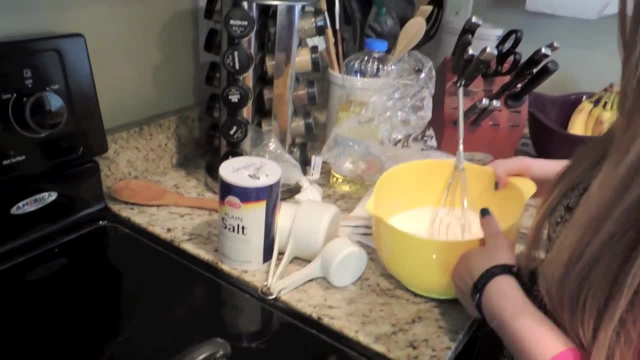 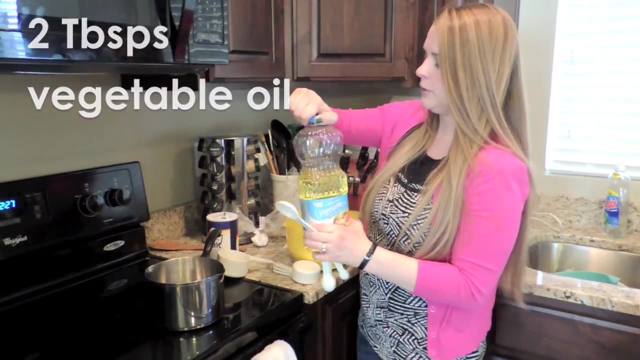 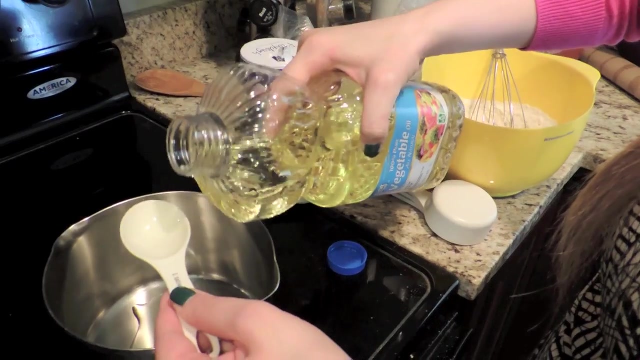 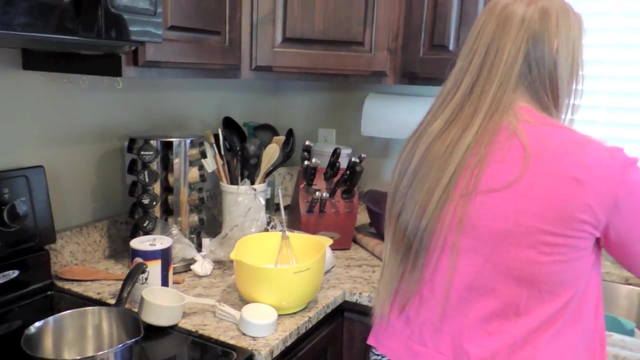 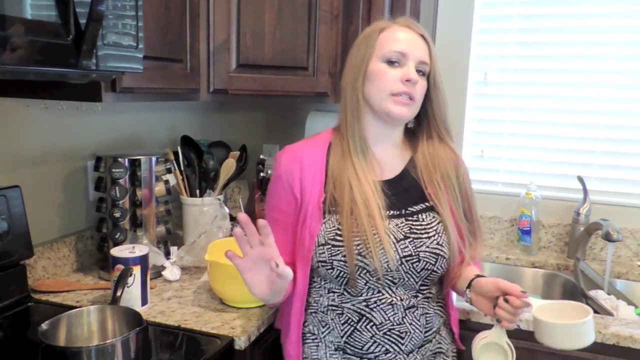 was bad: Mix, mix, mix, mix. Now you set that aside And here you put two tablespoons of vegetable oil, One, Two. At this point you would also add food coloring usually, But today I'm going to make a bunch of different colors, so I'm not going to add the food coloring. 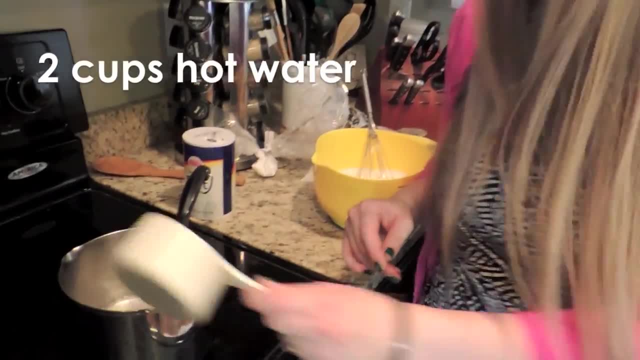 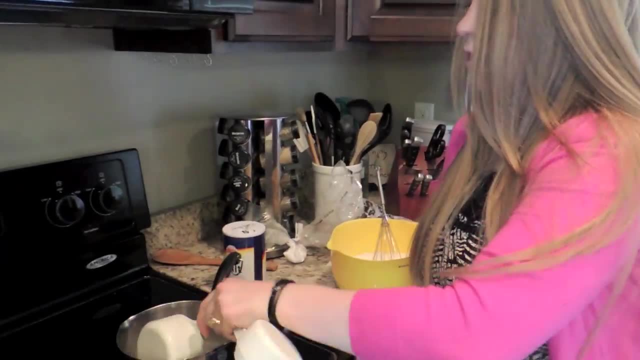 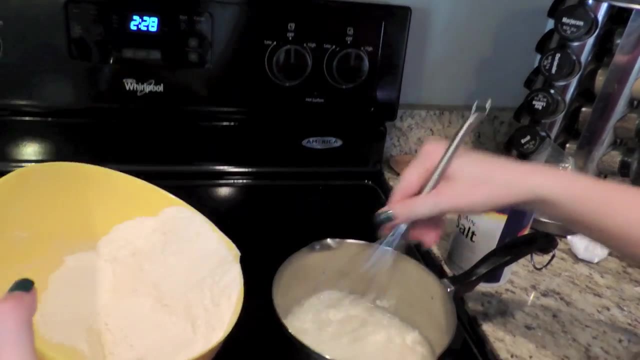 until the very end, You'll see. So one cup hot water is now all over my floor, And two cups hot water Now. I just add this stuff. I like to do a little bit at a time, at first Just kind of get that flour mixed in, And then I find it's a little bit easier. 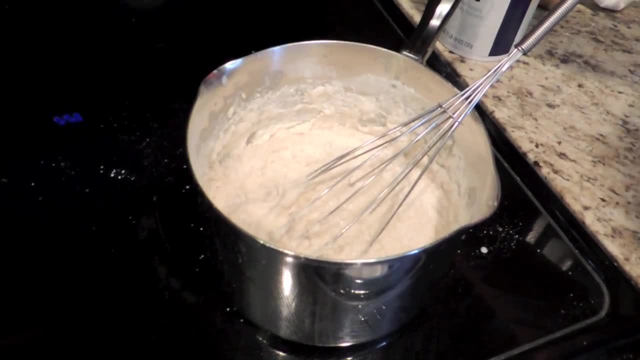 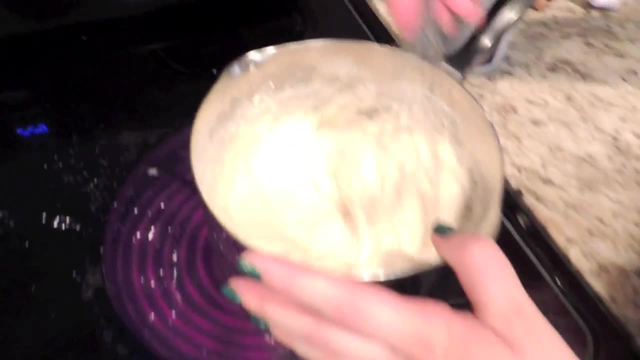 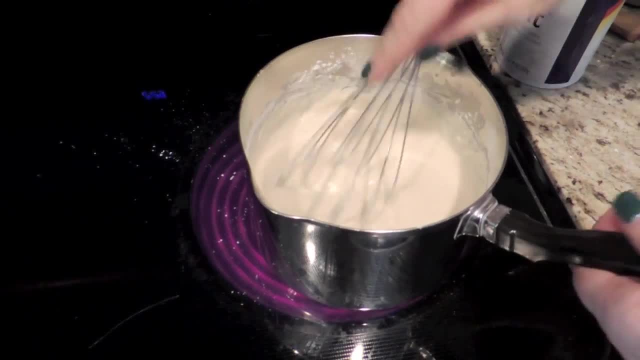 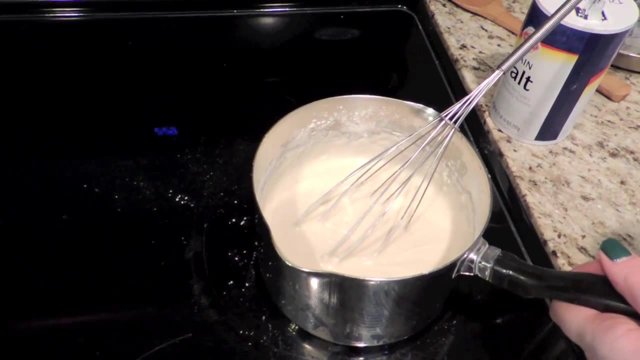 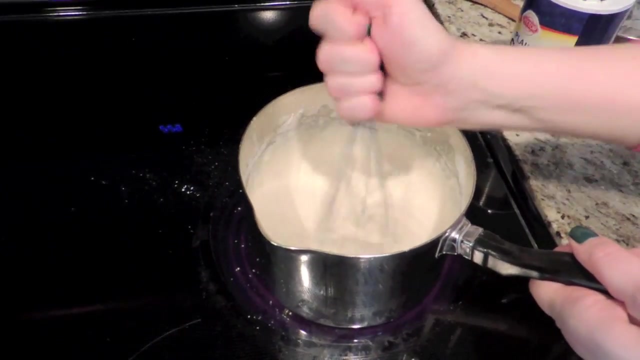 I keep using the um. what's this called The whisk? But as you can see well, right now it's not really like that. At first, if you see clumps it's just because your flour's not mixed in all the way. But once it starts heating up a little, you'll start to see clumps. 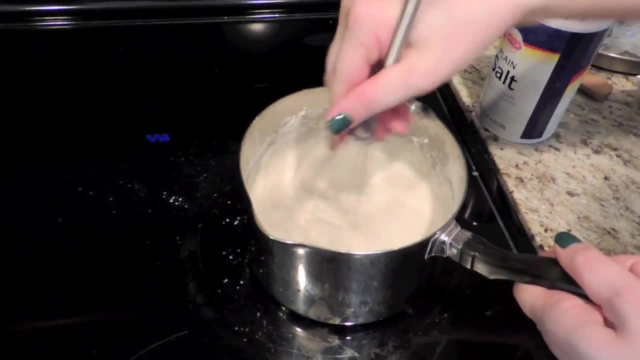 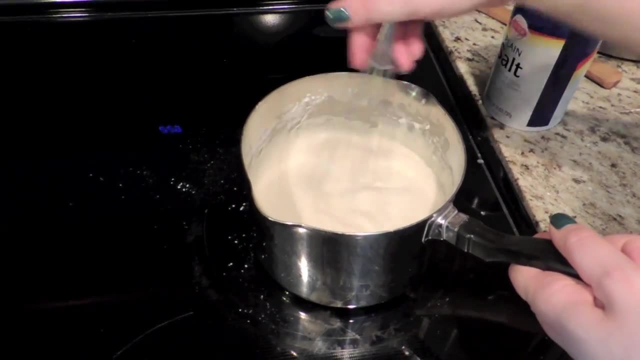 And it's just because your Play-Doh is hardening. It's getting harder, So. so at some point you'll have to switch to a different- um you know- spoon. Instead of using a whisk, switch to a spoon. Okay, you can see, I've switched to the spoon And the Play-Doh is. 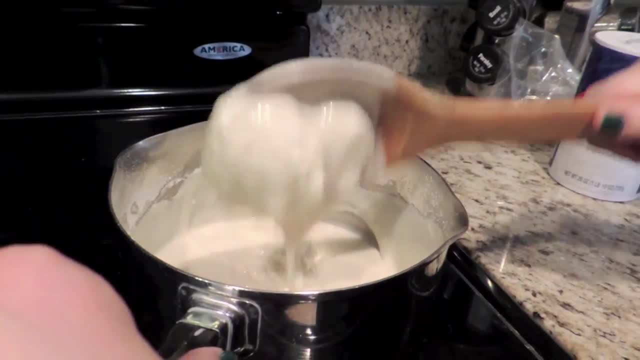 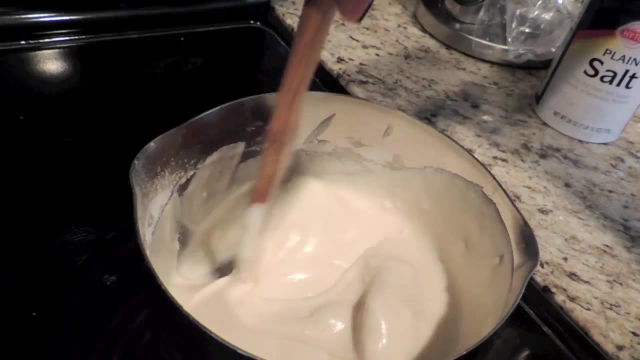 clearly sticking to it. So if that happens, just kind of get it off every once in a while And then just kind of scoop it. Make sure you're scraping the bottom, because that's where it starts to harden, is right against the bottom where it's hot, And just keep stirring. 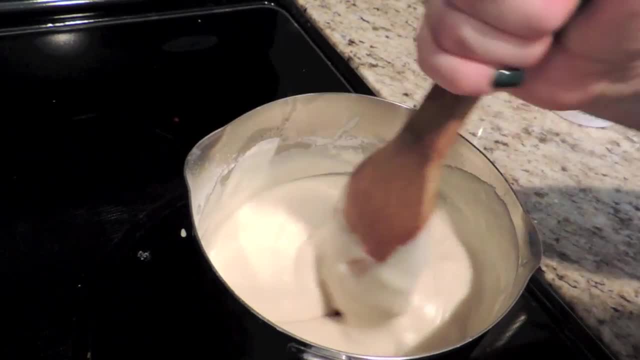 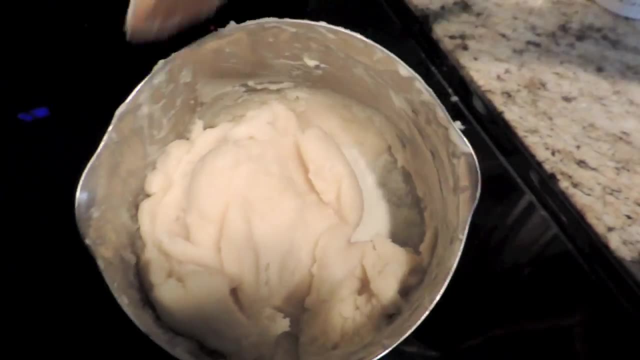 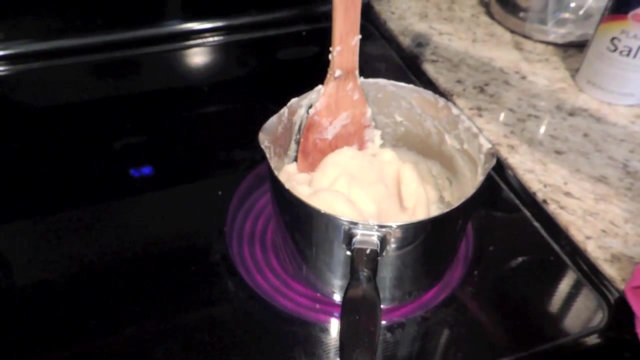 until it becomes more Play-Doh consistency. Okay, here we go. Now. it's pretty good. You can see the spots, the lighter spots, it's all pretty much cooked. So now I'm going to put this onto a piece of parchment paper to get ready to do the kneading. Okay so. 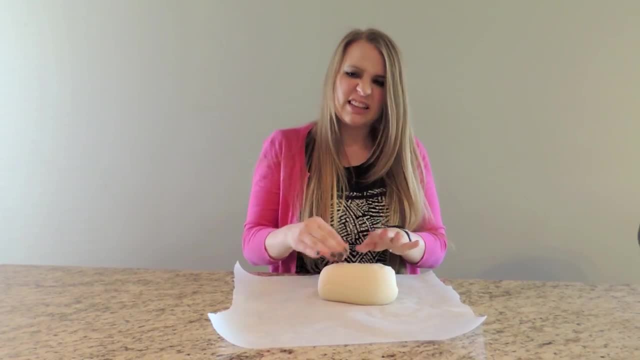 now I have my Play-Doh on here. It's pretty hot, So, um, you just need to let it sit for just a minute. Mine's been sitting for about a minute now, So now you knead it, uh, just. 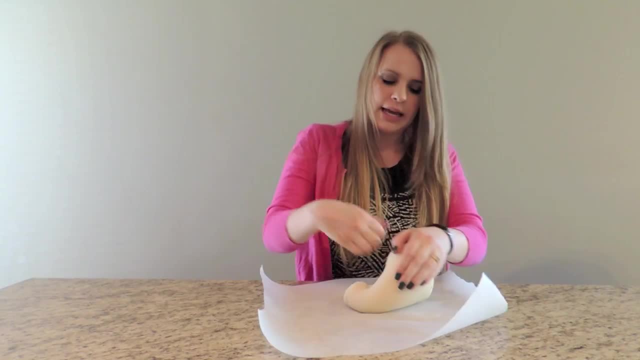 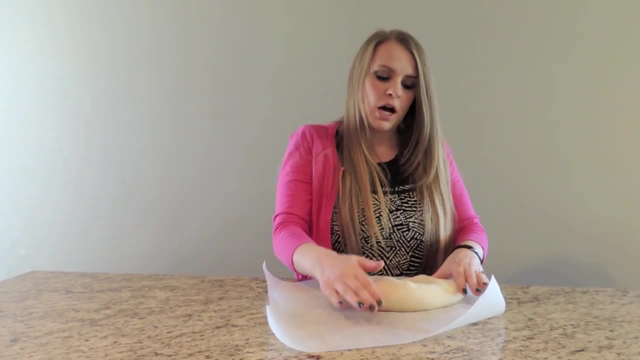 to get it really smooth, Get the same consistency all around and to get the nice uh Play-Doh texture that you want. And then, once I've kneaded mine just a little bit, we're going to add the colors. Now, as I said before, I usually do that at the beginning, But um, 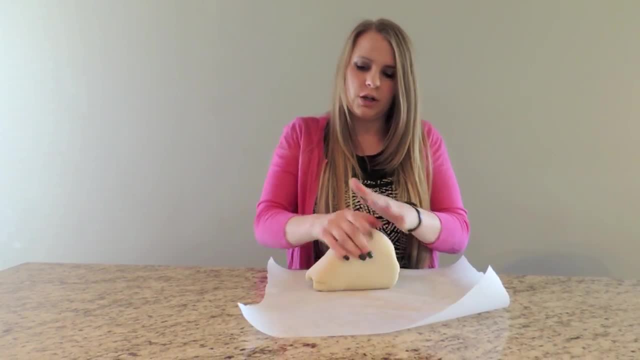 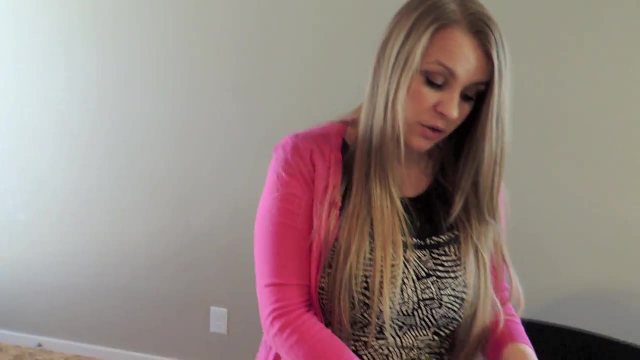 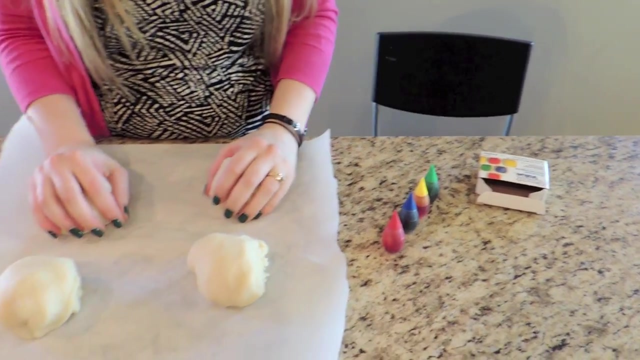 this time I'm going to do it right now, because I'm doing lots of colors instead of just one color. Okay, now I'm going to add the colors- Uh, these. we usually do a new Play-Doh every month, So this is our April Play-Doh, And I'm just going to do some spring colors to. 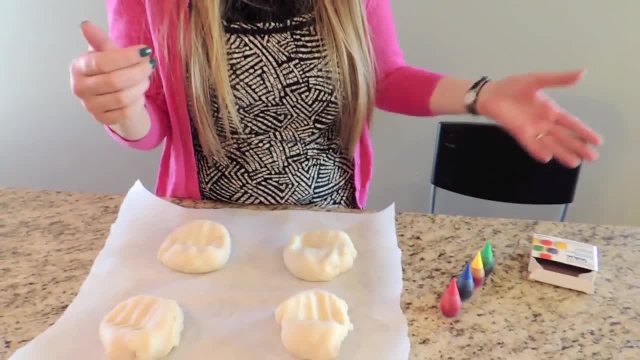 make them really pastel. So I'm just going to do four colors, just these colors. but they're going to be pretty cool, So I'm just going to do four colors. So I'm just going to do three of each. If I were to have to use my noses and then I take it out, it's.